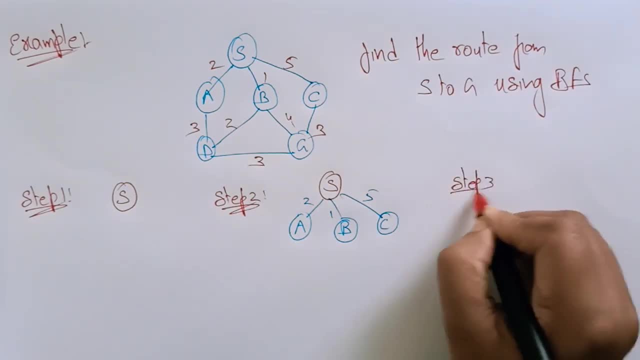 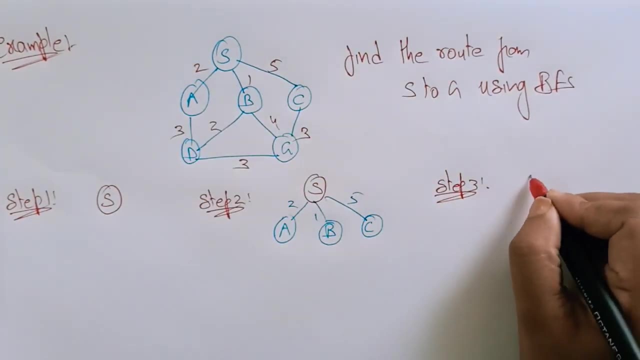 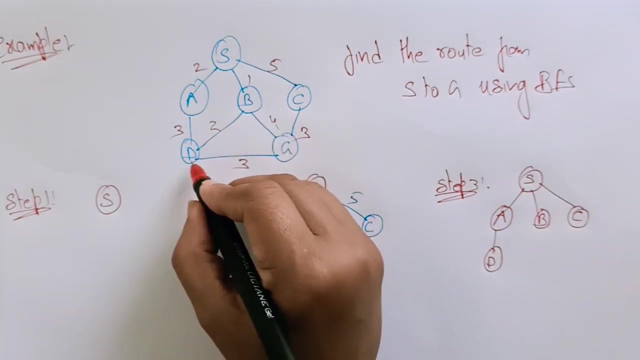 Now coming to the sorry step 3.. So in the step 3, expand the graph. Expand the graph in the form of a tree, Just expand it. S is the root node, A, B, C are the successors And again in the next level, A successor is the G and B successor are the D and G. D and G And C is connected to G. 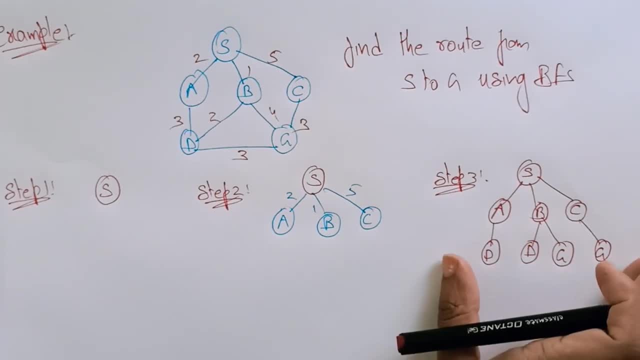 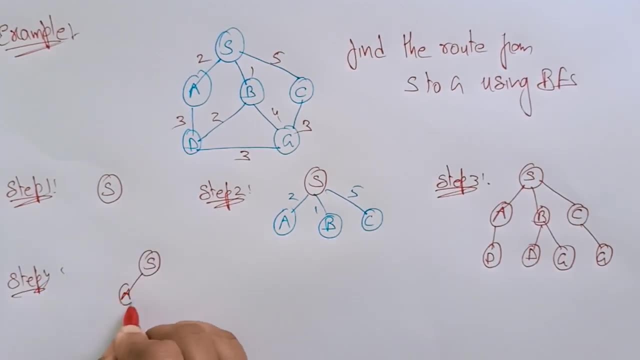 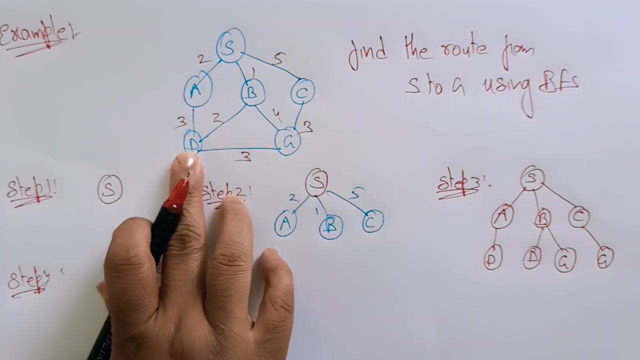 Okay, Still, I need to expand. It is not completed, So expand Step 4.. S, A, B, C. Now A is connected to D, B is connected to D, as well as G And C is connected to G. Again, this D is connected to D is connected to G. 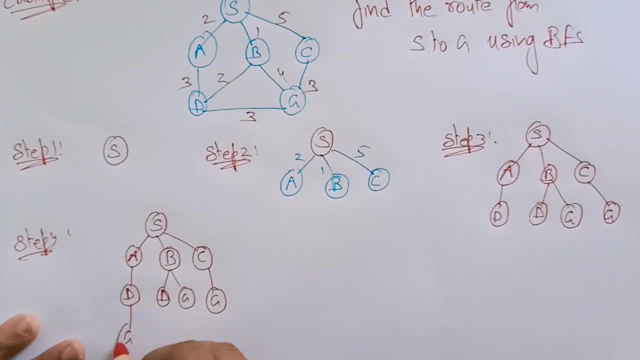 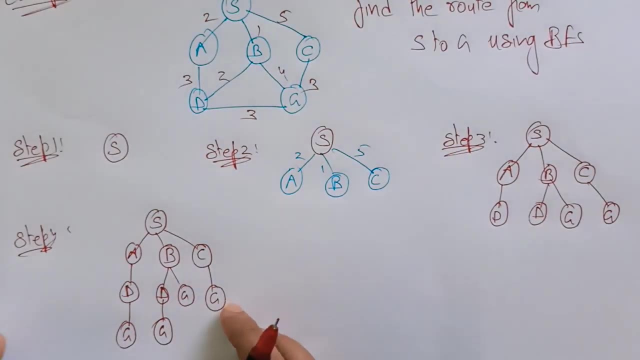 So wherever the D is there, you just Expand it. So this is the way you get the tree. Okay, The given graph. I expanded it and it is formed in the tree. The weights are 2,, 1, 5.. 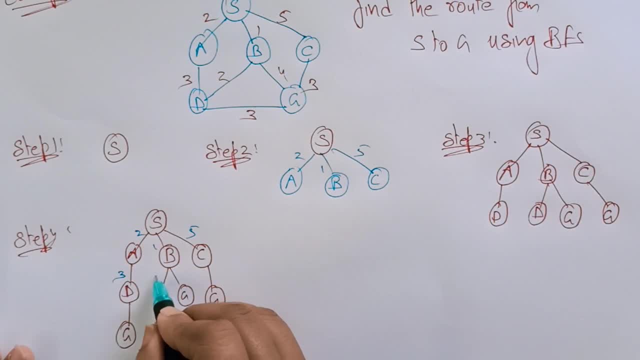 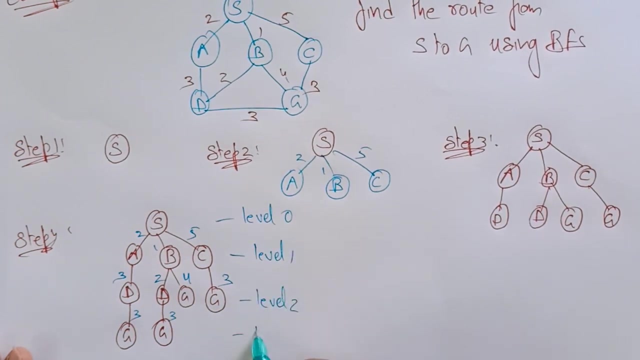 This is 3.. And this is 2,, 4,, 3.. This is 3 and this is 3.. So this is at level 0 and level 1. And level 2.. And this is level 3.. 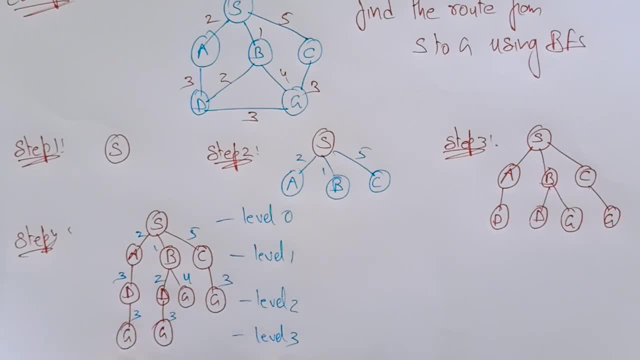 Okay, So up to this is the level 3.. So now I want to answer Means. I want to find the root from S to G. So which path I need to be take? I have to choose using the breadth first search. So what is the breadth first search? 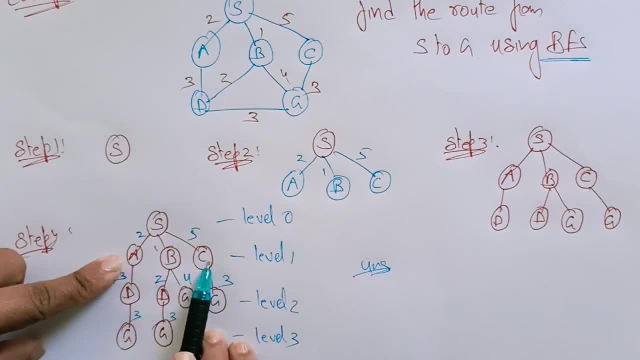 You have to visit all the successor in that level, Means all the nodes in that level. Okay, So the path in the second depth. So here, in this second depth, you will get your solution, because here the g is there. okay, so the path.